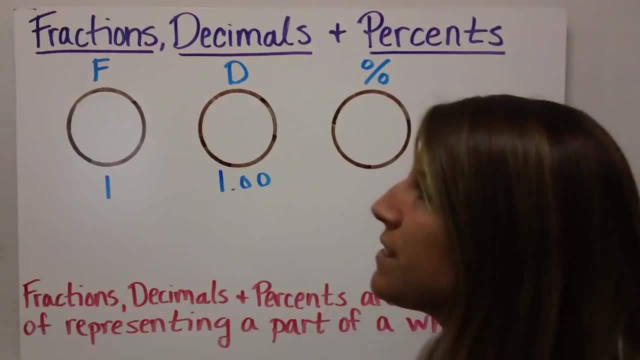 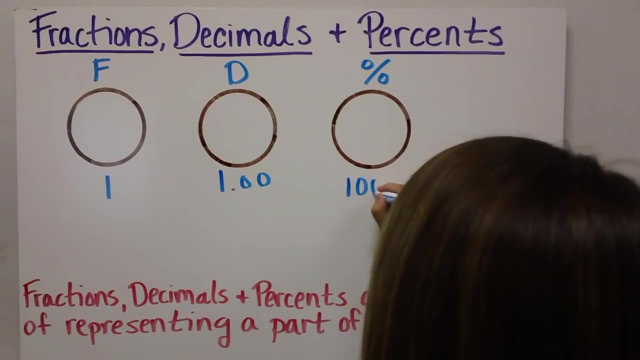 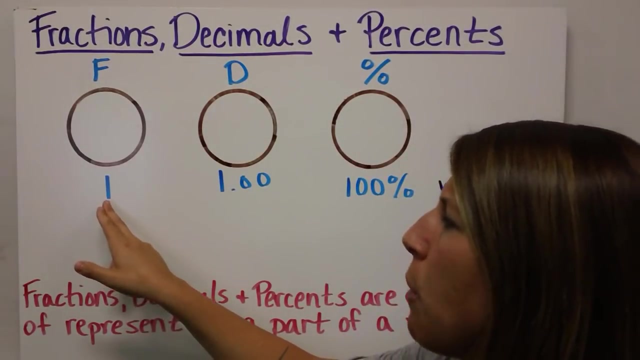 is if you have one whole and we're talking about the percent. a percent is not one percent, it's one hundred percent. So that's how we represent the whole as a percent, and I want you to think about how do we get from one to one hundred, And each of them are talking about the same amount. 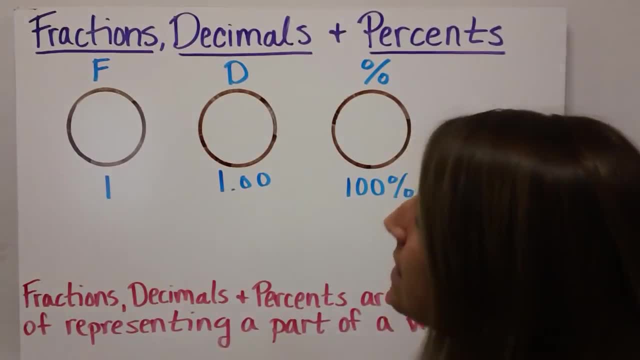 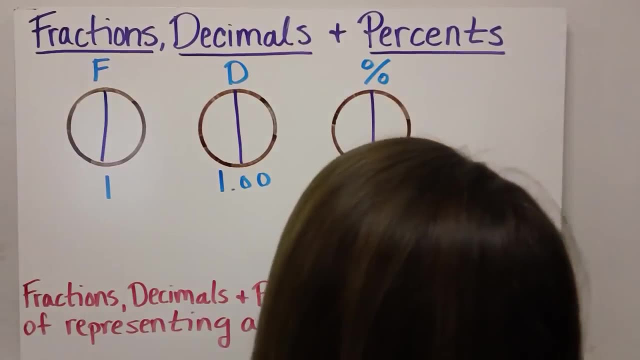 of a whole, so that's very interesting. Now I'm going to take each of these and divide them. I'm going to divide them right down the middle and they're not going to be super accurate, forgive me. okay. What I've done here is I'm going to say, okay, I've broken. 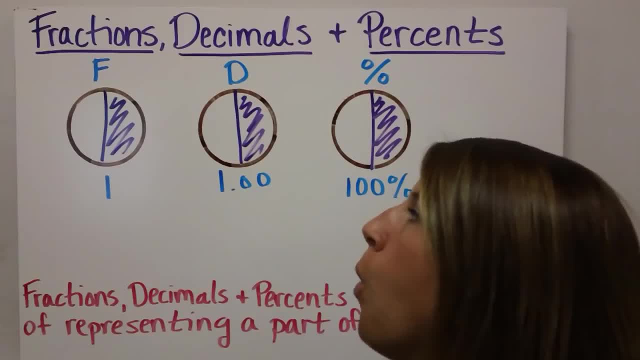 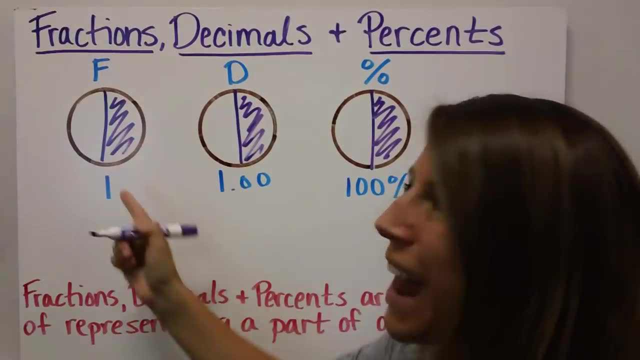 them all up. I've got a bunch of zeros, I've got a bunch of zeros and I've got a bunch of zeros and a bunch of zeros. So I'm going to divide them all up the same way. What is this as a fraction? 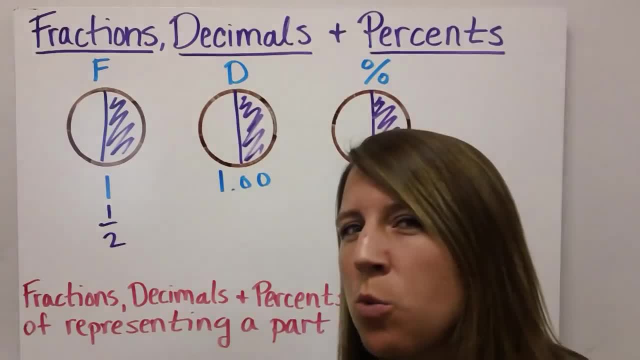 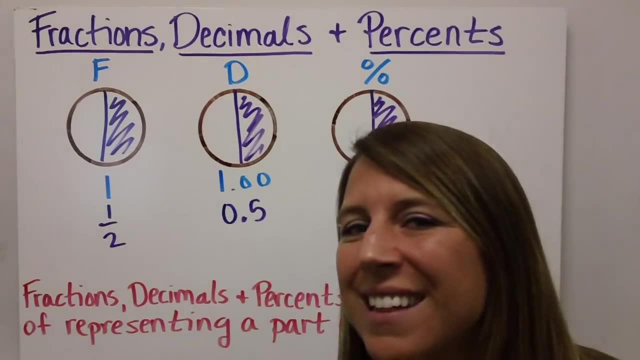 Should all be something that you're relatively familiar with. Well, this is one half. so as a fraction I can represent that as one half. How about as a decimal? How do we represent one half as a decimal? Five tenths. so that's zero point five. But what about as a percent? 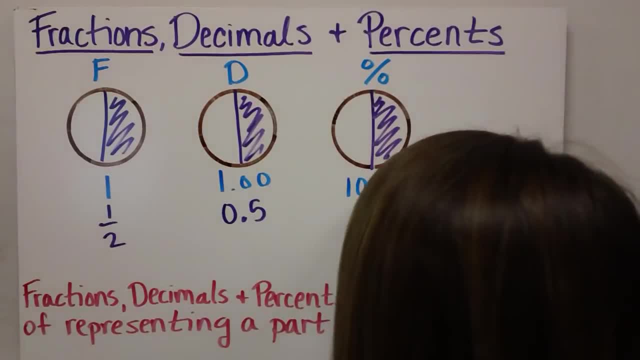 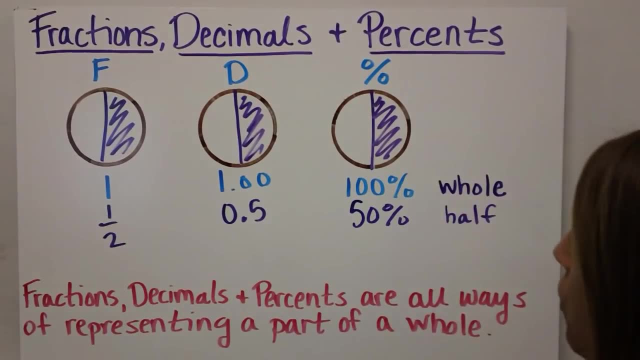 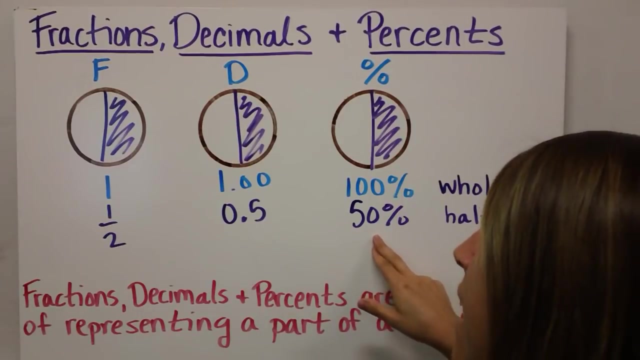 Most of you are going to know that that's fifty percent. Okay, and in all three of these cases we're talking about one half Interesting. One half is five tenths as a decimal. five tenths is fifty percent as a percent. How about moving from one to one hundred from? 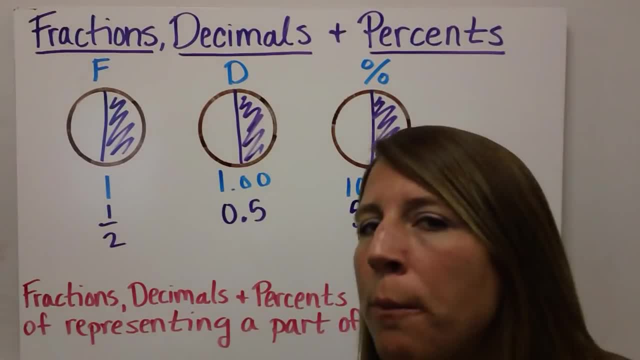 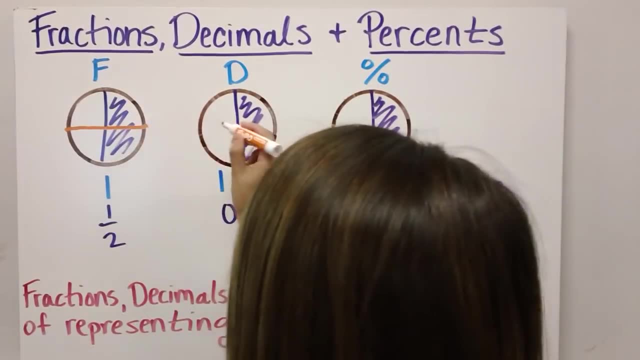 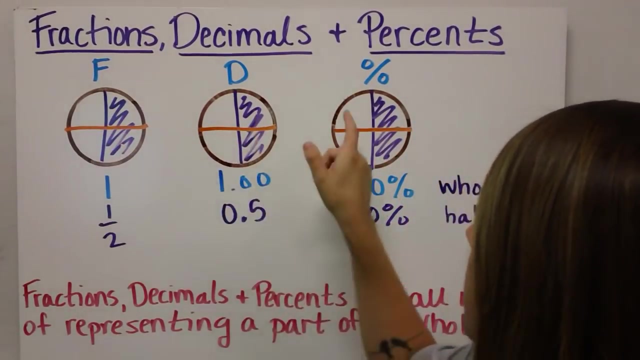 five tenths to fifty, numerically, We're going to do one more. I'm going to divide this yet and I'm going to say this: Now, each of these holes have four equal parts. Okay, that's the way we're going to look at this. If I color in and I 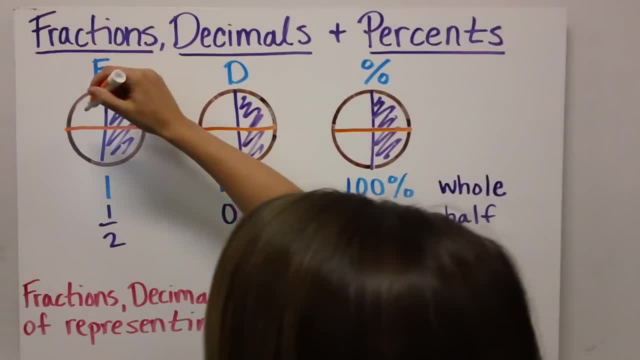 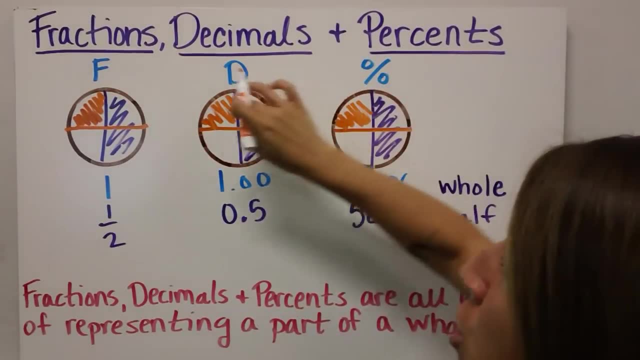 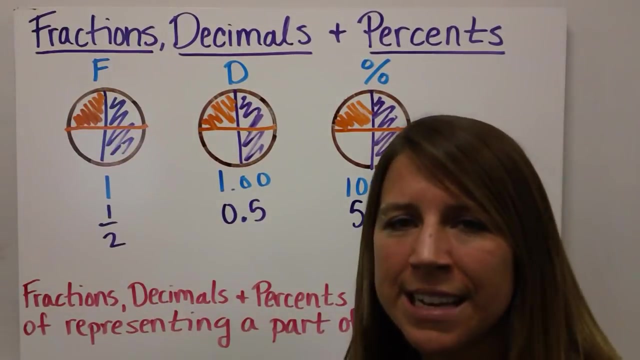 just want you to look at the orange sector. If I color in this piece right here now, just focus on the orange piece now. how much of the hole is that? How much of the hole? Four equal pieces. that orange piece is going to be one fourth right, One fourth. 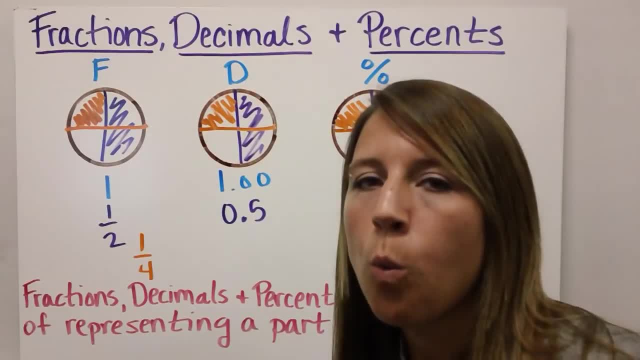 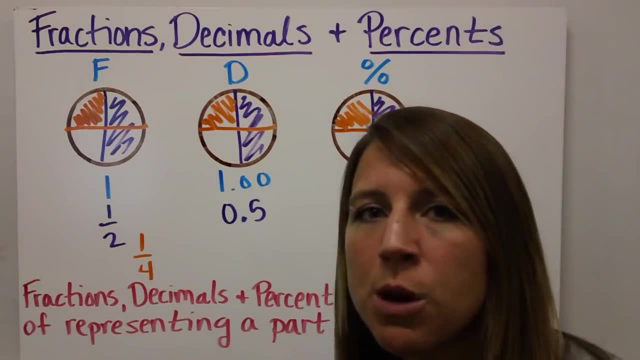 And we can also say one fourth as one quarter. That helps me when I think about the decimal version. One quarter- most of us are probably pretty comfortable with saying: well, a quarter, that's like 25 cents. I know how to represent that as a decimal. 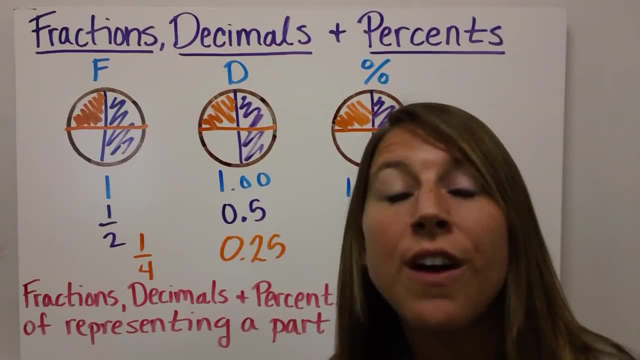 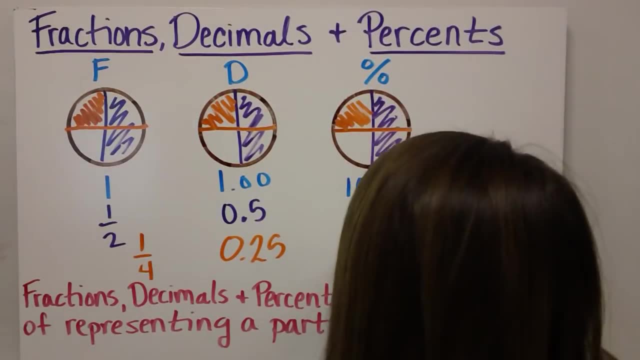 0.25 or 25 hundredths. 25 hundredths is like 25 cents related to money, And then, as a percent, one fourth is 25 percent. It's very interesting, And then here we're working with a quarter. 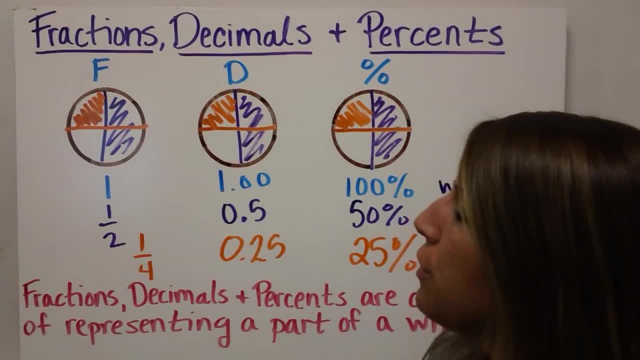 So I want you to focus on the relationships from the decimal to the percent. How are we getting from here to here? How are we getting from five tenths to 50?? How are we getting from 25 hundredths to 25?? 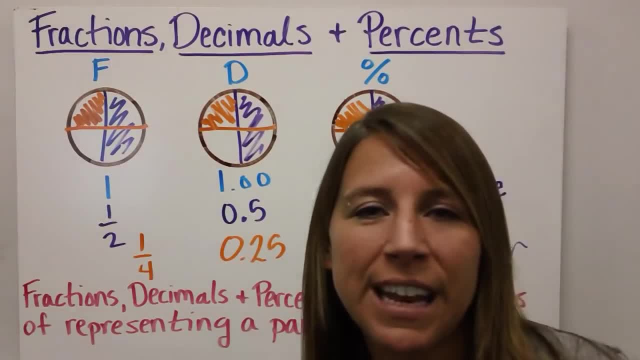 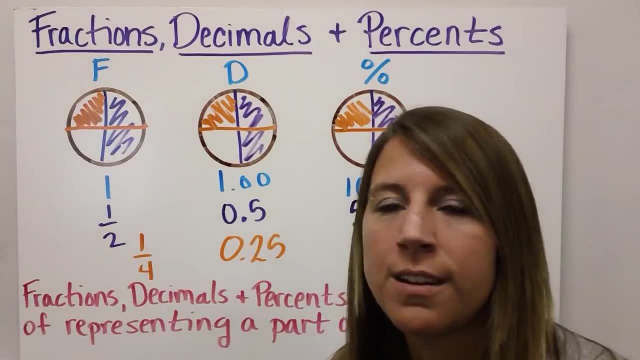 Well, how do you numerically and think multiplicatively, get from 1 to 100?? You don't add 99,, I'm not talking addition. Multiply by 100.. Multiply by 100.. From 1 times 100, do I get 100?? 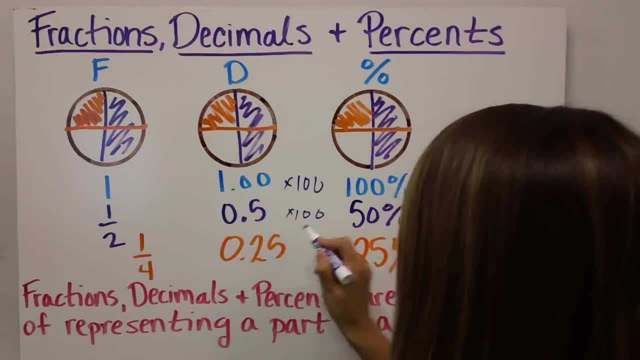 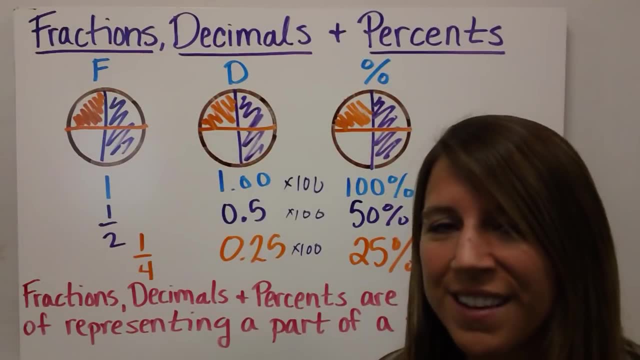 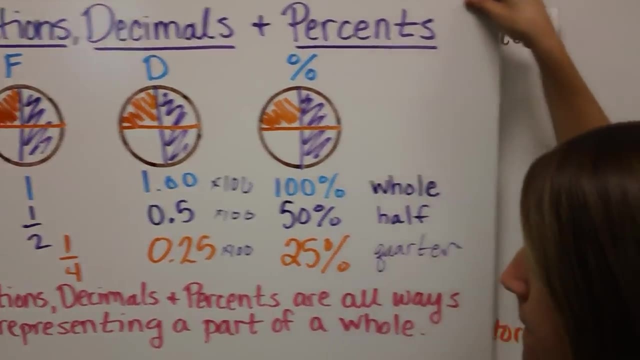 Yeah, How about 5 tenths times 100?? Sure enough, I'm going to get 50.. 25 hundredths times 100 is going to give me 25.. So that's how decimals and percents are related. Now here's. 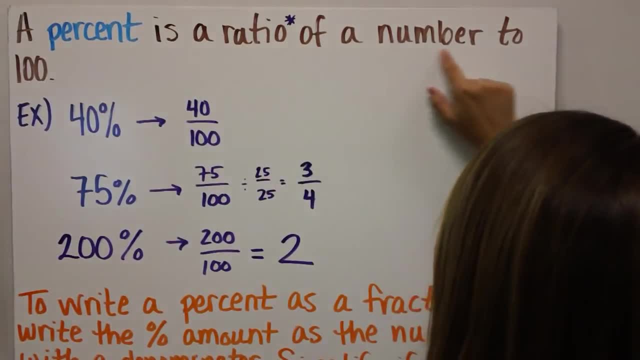 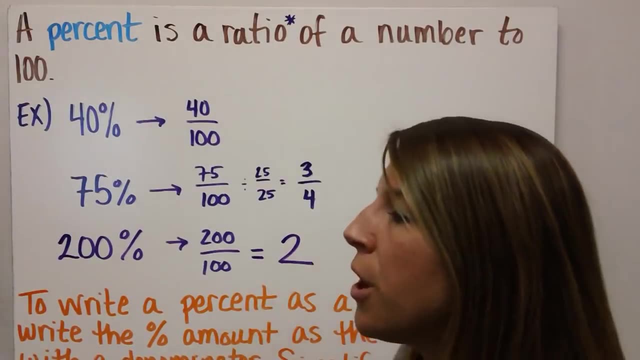 the definition of a percent. A percent is a ratio of a number to 100. A ratio which we may have gotten to already or we will get to later. a ratio is a comparison of two numbers by division And we like to look at. 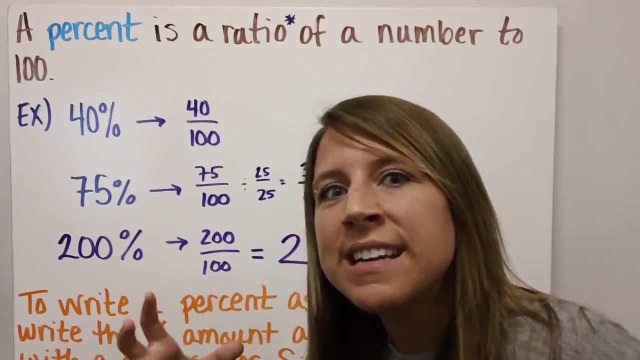 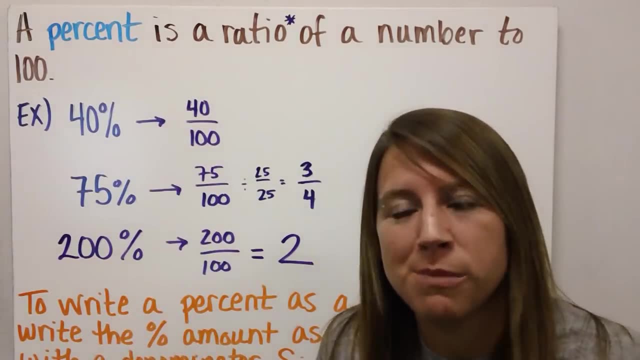 division with fraction bars. So you're going to see a lot of comparisons among ratios, percents, fractions and division. They all kind of fall in the same realm. It's really cool how we can connect all of those concepts together. So again, a percent is a ratio. 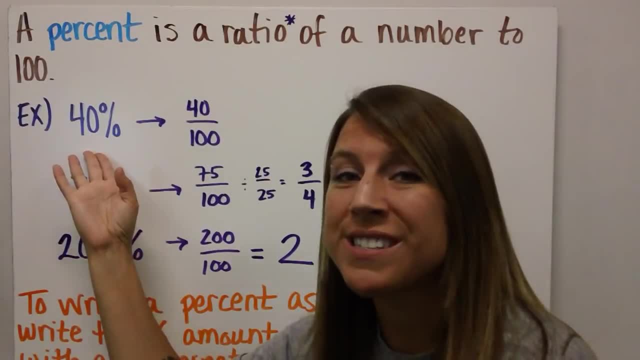 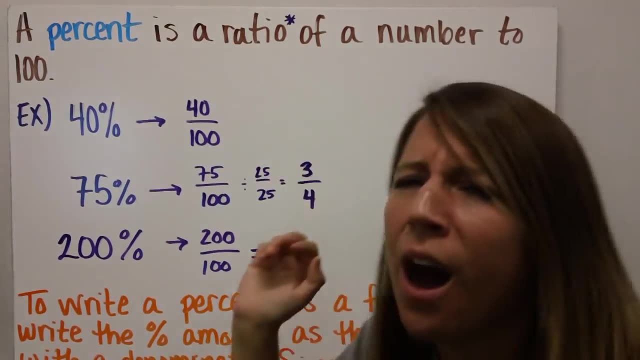 of a number to 100.. So if I was talking about 40 percent, we would write that and could write that as 40 to 100, or 40 over 100, or 40 hundredths, 40 hundredths. 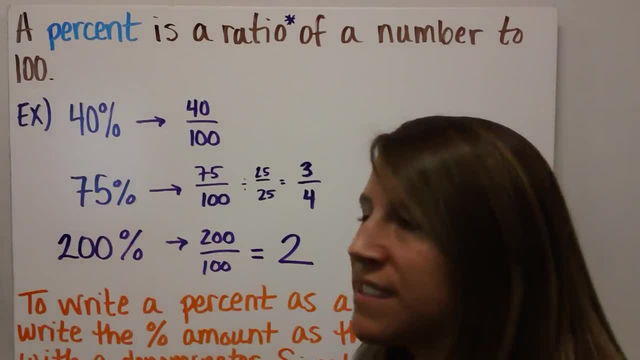 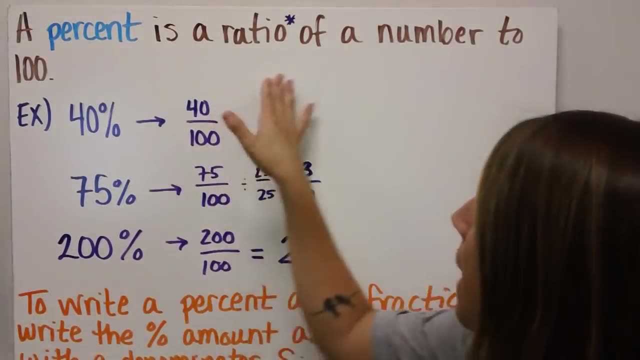 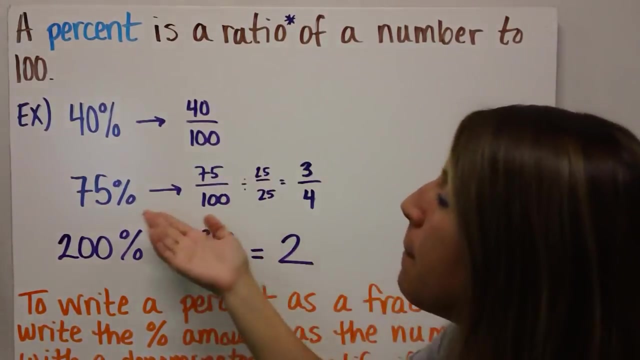 is 40 percent. 75 percent can be written as 75 hundredths. 200 percent can be written as 200 hundredths. It's a comparison of a number to 100,. okay, by division. So if we come back to 75 percent, here we know. 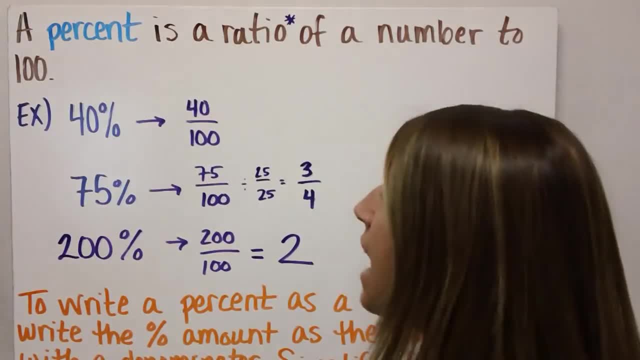 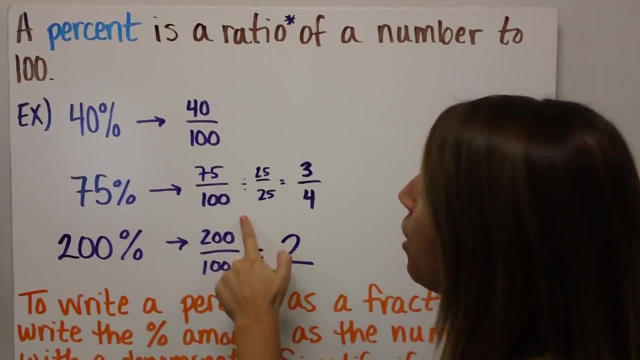 that 25 percent is 1 fourth as a fraction. I wanted to show you here that, because I can write 75 percent as 75 hundredths, if I simplify 75 hundredths that to me is 3 fourths, And how perfect sense does that make? 3 quarters. 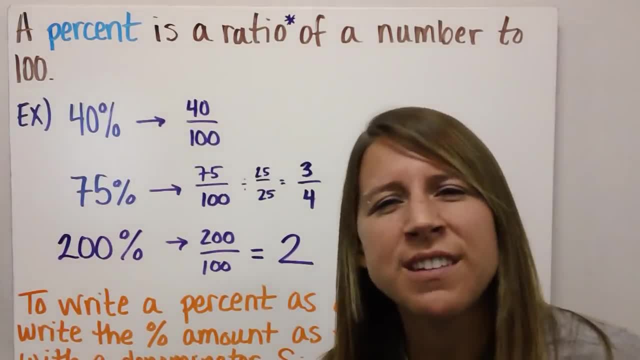 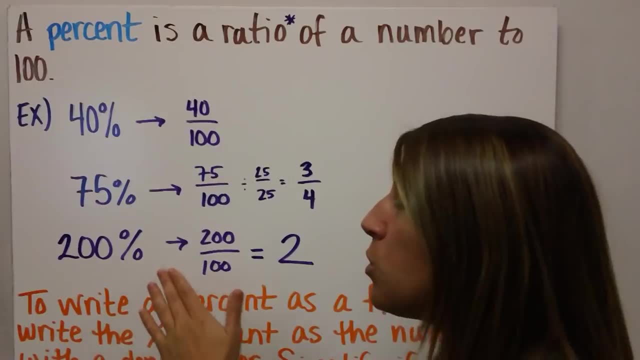 is 75 cents. 75 cents is 75 percent of a dollar. All sorts of links there that can help you understand how percents work. 200 percent- Well, 200 percent is more than 1 whole right, Because 1 whole is 100 percent. 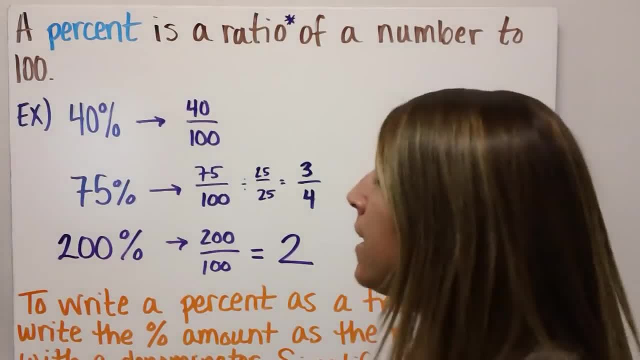 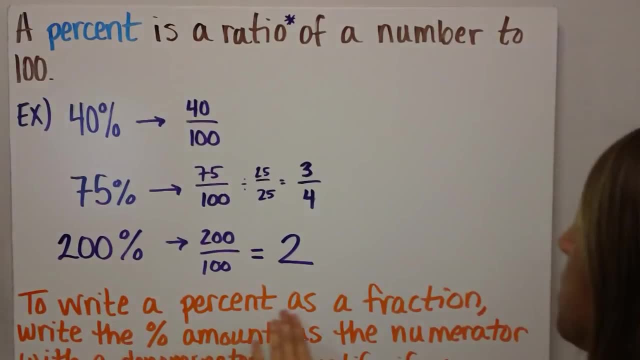 So 200 percent. it makes sense that it would be more than 1, because 200 hundredths simplifies to 2.. Right, So to write a percent as a fraction, you write the percent amount as the numerator, with a denominator of. 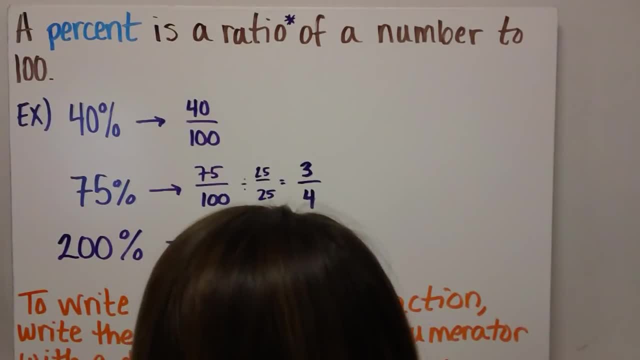 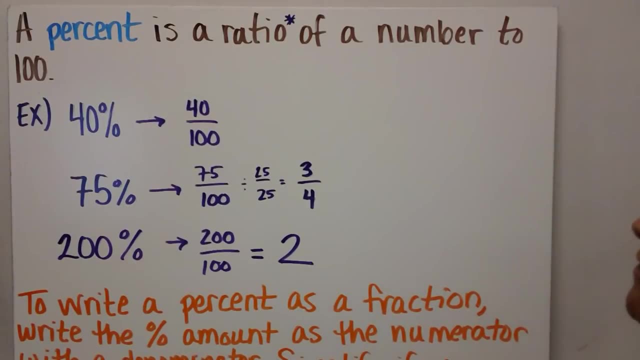 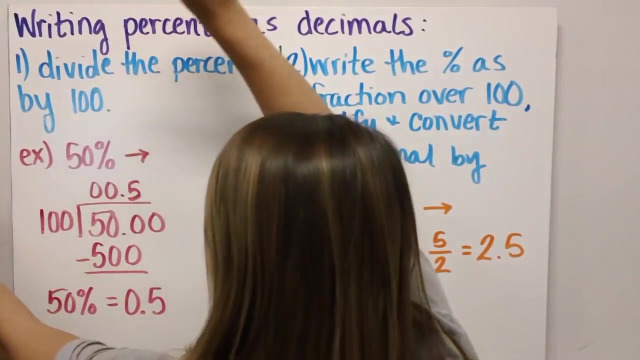 100.. I missed that. It's the denominator of 100. That goes here. Period. Okay, Then simplify if necessary, and I've kind of gone through that up here for you. Alright, So there are lots of methods to changing. 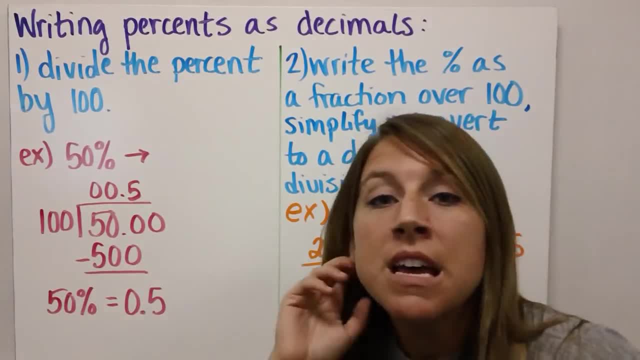 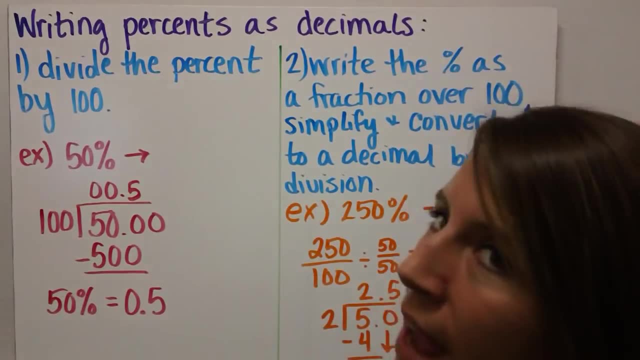 percents to decimals, to fractions, and moving among them. There are lots and lots and lots of ways to do that. I'm going to give you as simple as ways as I can. So first, writing percents as decimals. Some of you may already know. 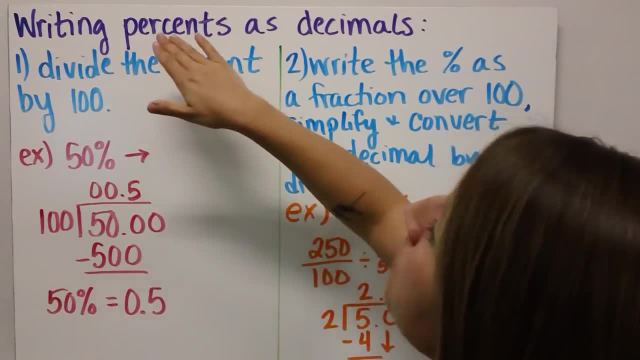 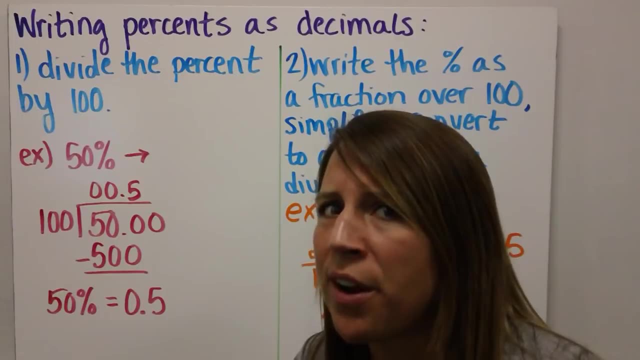 a shortcut, but I want you to think of why that shortcut works. As we learned in our first board, to get from percents to decimals, there's that multiplicative 100 in there, isn't there. So to get to go from a percent to a decimal then, 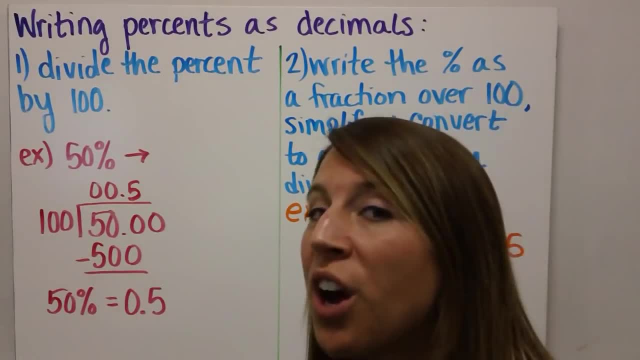 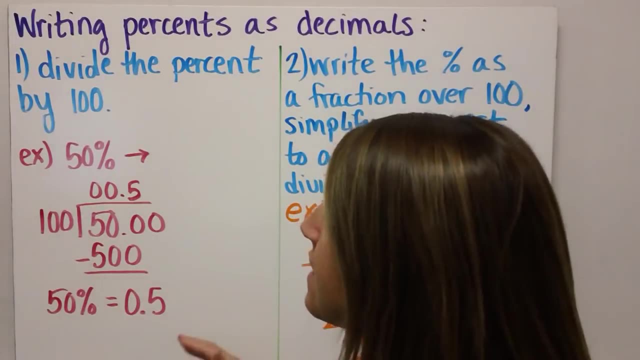 you take that percent and you divide by 100.. So if I had 50%, what is 50% as a decimal? Well, we've already worked with that, but to prove it I can say: well, 50%. 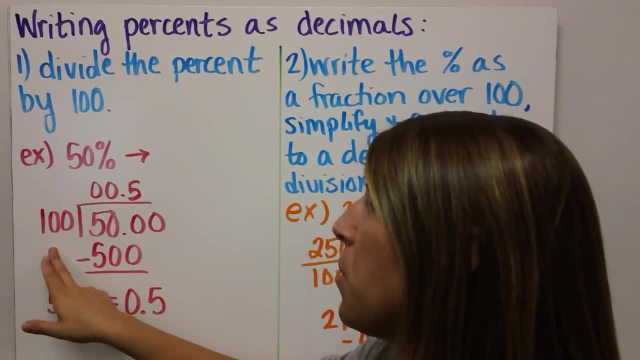 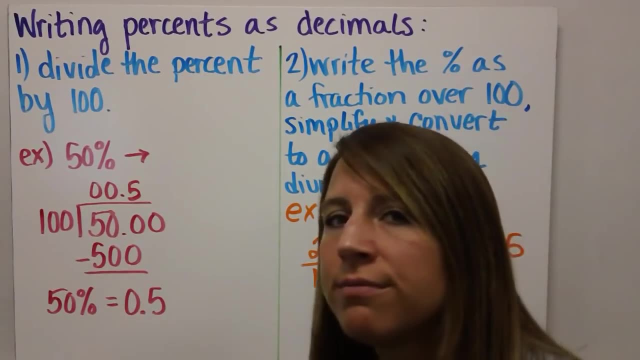 I'm going to divide 50 by 100.. 50 divided by 100, I have to add my decimal points. 100 goes into 500 five times, and then I'm left with 0.5.. 5 tenths equals. 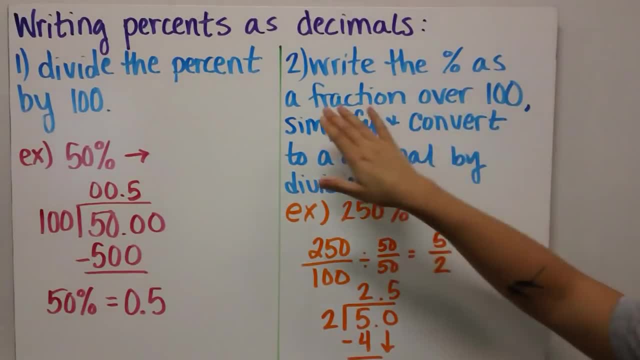 50%. Another way is I can write the percent as a fraction over 100, then simplify and convert it to a decimal by division. So for example, 250%. we know that that's more than one whole, so keep that in mind. 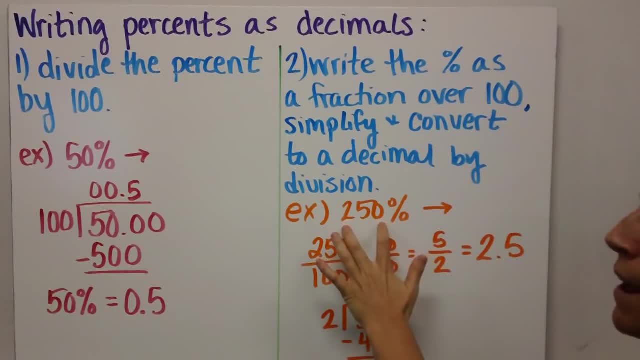 250%. well, I know, any percent is a comparison to 100, so I can write that as a fraction And then I can simplify. This is just dividing by 1 here, so I'm not changing any values. 50 goes evenly into both. that's why I do 50 fiftieths. 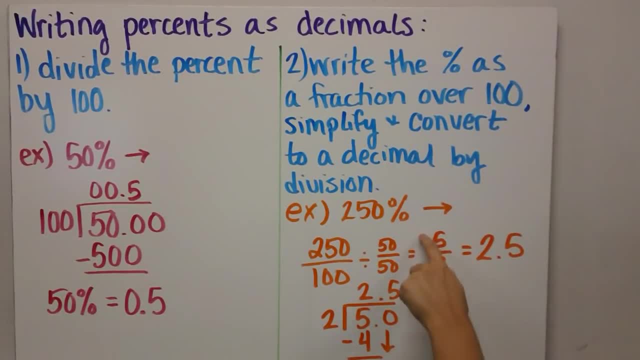 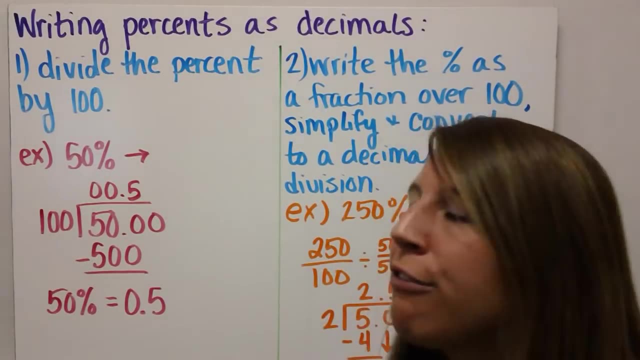 I get down to 5 halves and I can say: well then, I can just divide 5 by 2.. 5 divided by 2 comes out to be 2.5, or 2 and 5 tenths 2 and a half, 250%. 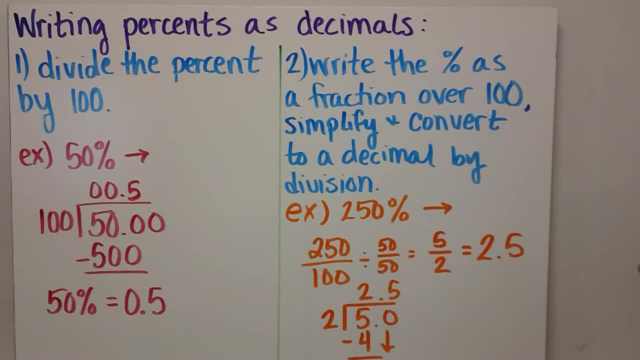 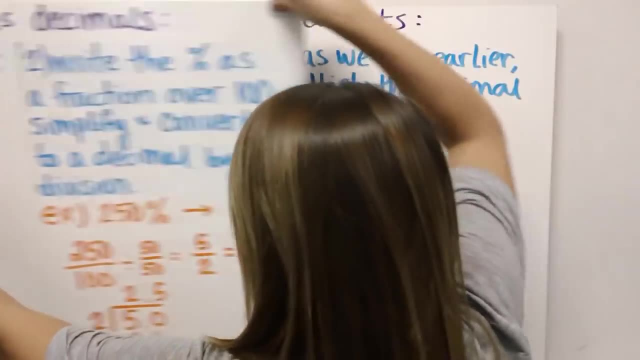 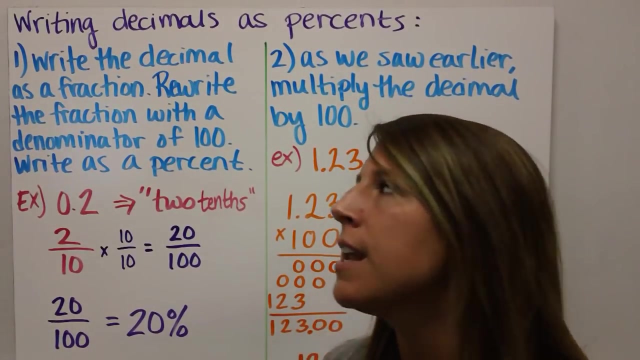 is the same as 2 and 5 tenths- Excuse me- is equal to, not the same as. Oh man, my boards are falling Writing decimals as percents now, so this is going in the opposite direction. If to write a percent as a, 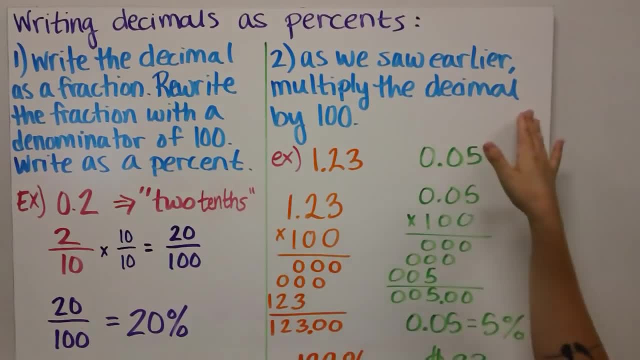 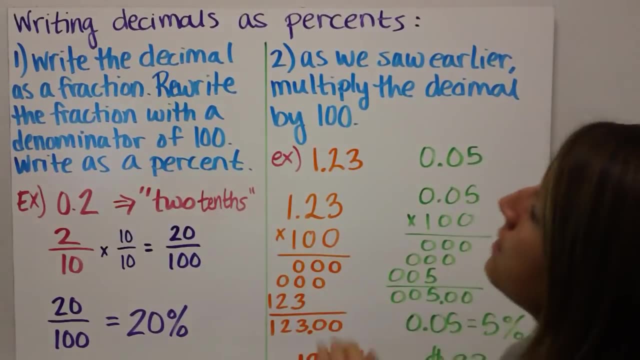 decimal, we divide it by 100, then we can multiply by 100, just the opposite here, to get to a percent from a decimal. So I'm going to do this one first. If I have 1 and 23 hundredths and I want to know what that is as a percent, I can just multiply. 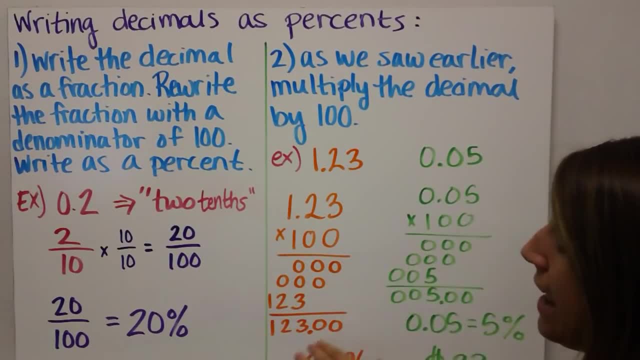 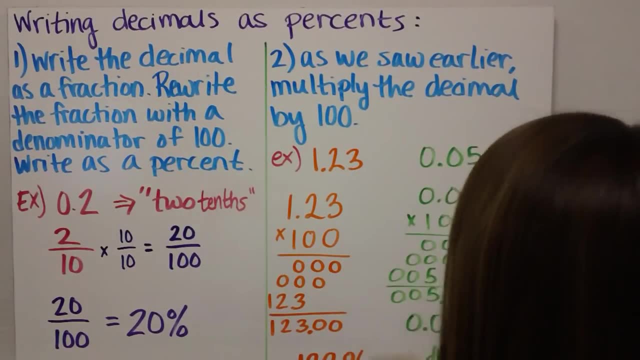 by 100. Here I've done the math the long way and I get 123, so that's 123%. If I have something else to think about, that I've kind of hit on earlier. here's 5 hundredths, 5 hundredths as a percent. well, I multiply by. 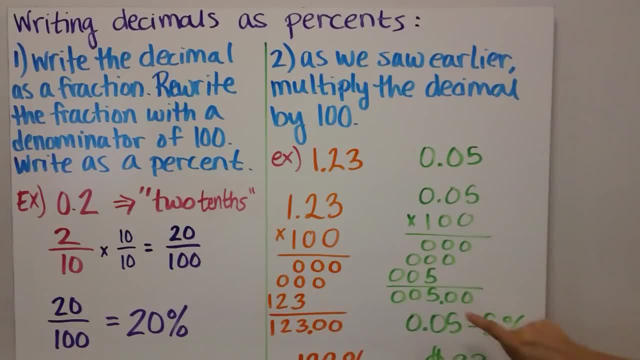 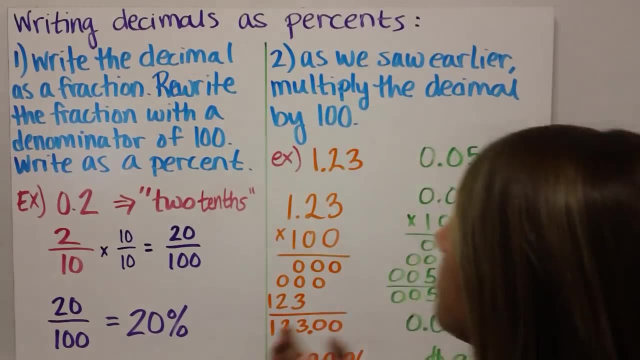 100, and I get 5 percent. 5 percent, How does why does that make sense? Relate that to money for a second. If you have 5 cents, which is what this looks like, right? If you have 5 cents, how, what percent of a dollar do you have? 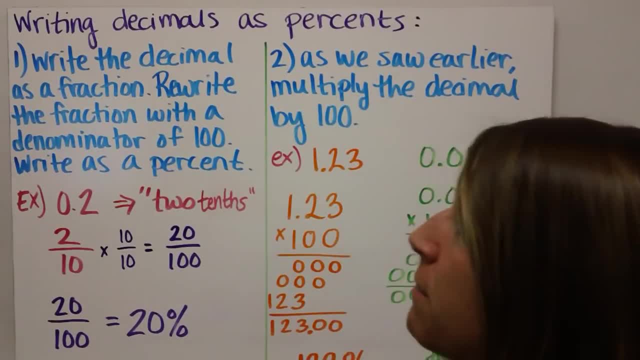 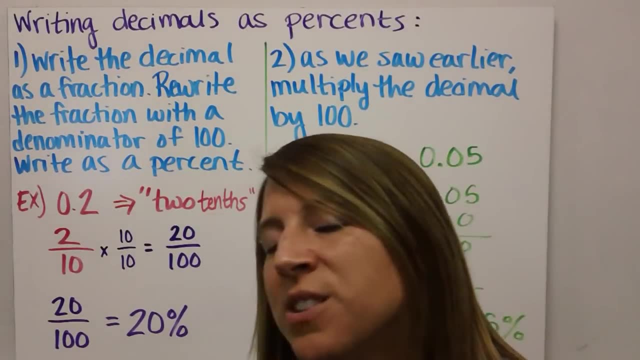 5 percent of a dollar. It's interesting, right? You can also write the decimal as a fraction, then rewrite the fraction with the denominator of 100 to write as a percent. It's kind of a longer way, but if you're more comfortable then you can do that. So, for example, if I had 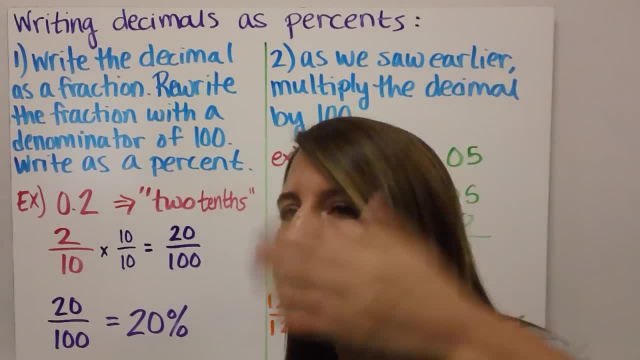 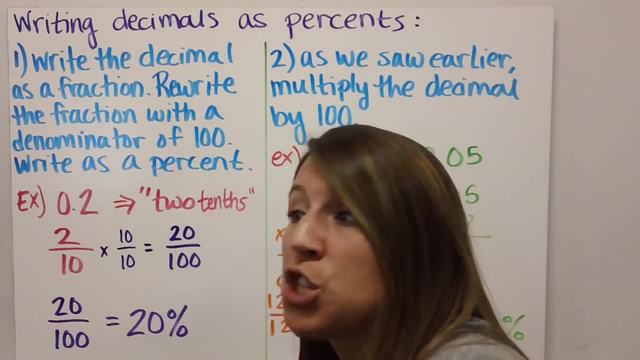 .2, two-tenths, two-tenths, that's two tenths, so I can write it as a fraction. but this doesn't have a denominator of 100, so I cannot say that that's 2 percent, because I can only say that if I had a denominator of 100.. But if I multiply by 1, 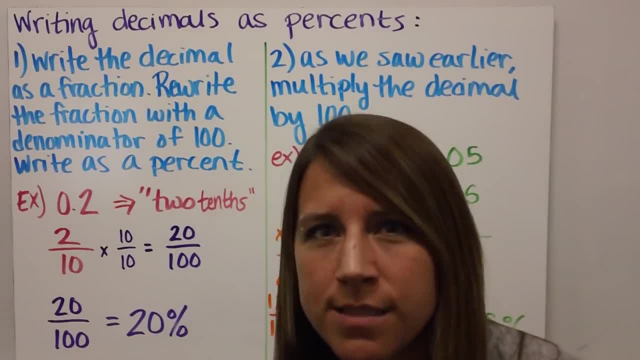 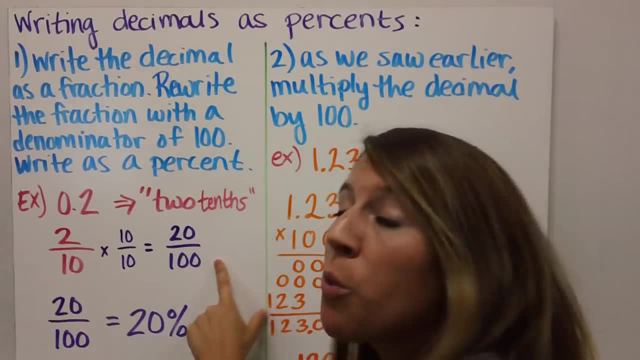 here and you might be saying: well, that's 10 tenths. 10 divided by 10 is 1, so I'm technically just multiplying by 1.. I keep the value. this is 20 hundredths, Now that it's over 100, comparing to 100. 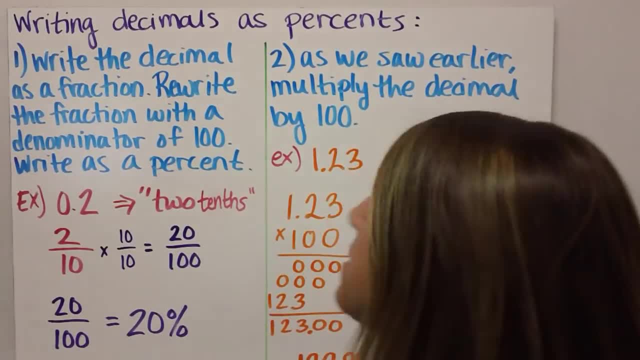 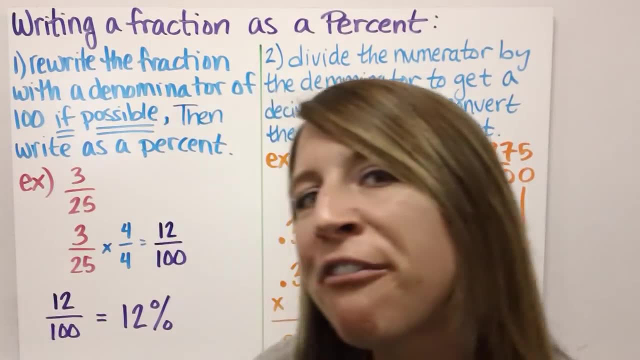 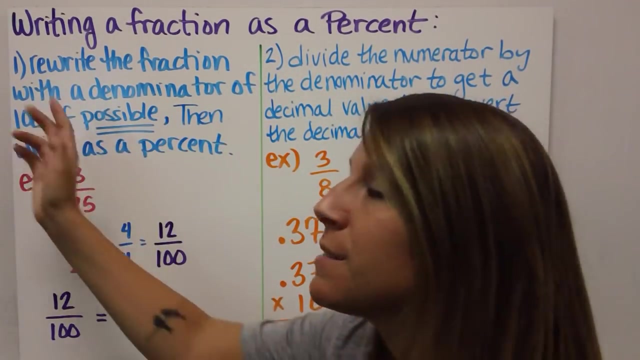 I can say: well, that numerator is my percent, 20 percent. How about writing a fraction as a percent? You can. here's one thing you can do. you can rewrite the fraction with the denominator of 100, if possible, like we just did on our previous board here. 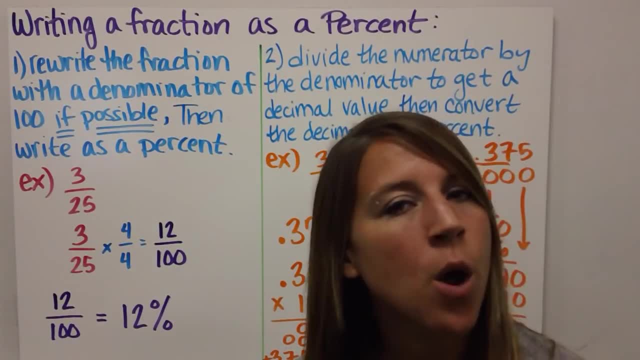 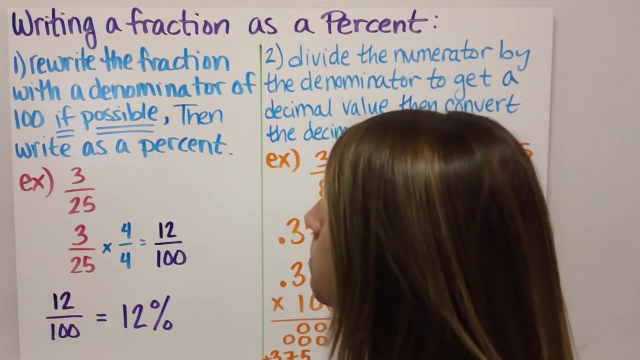 Then write as a percent, And this is only if possible. it's not always going to be possible. Your denominator must be a number that goes evenly into 100 for this to work. If I have 3, twenty-fifths immediately, I know 25 goes into 100 evenly. 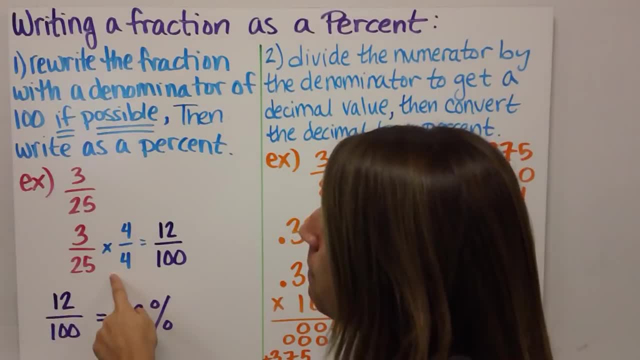 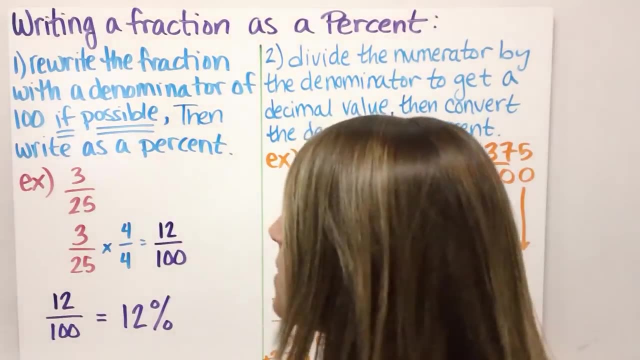 So if I rewrite this fraction by multiplying by 4 fourths, I get 12 hundredths. 12 hundredths is equivalent to 3 twenty-fifths and because it has a denominator of 100, I know that 3 twenty-fifths is equivalent. 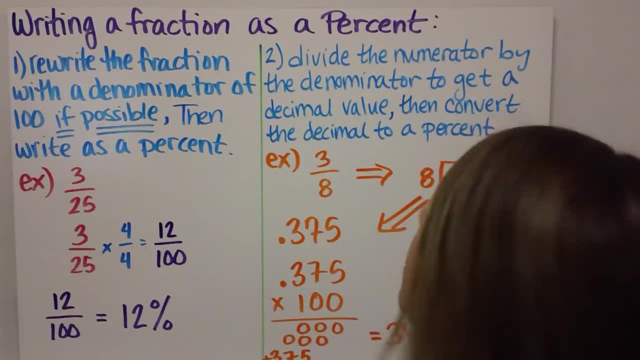 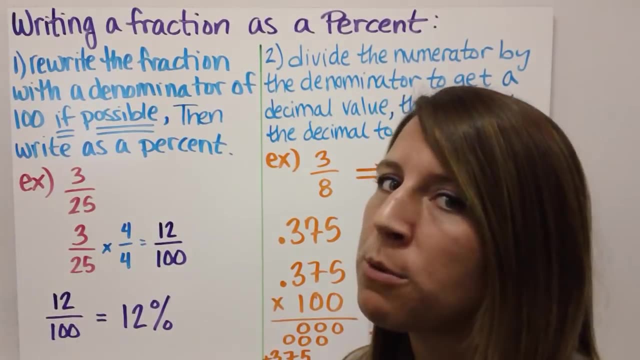 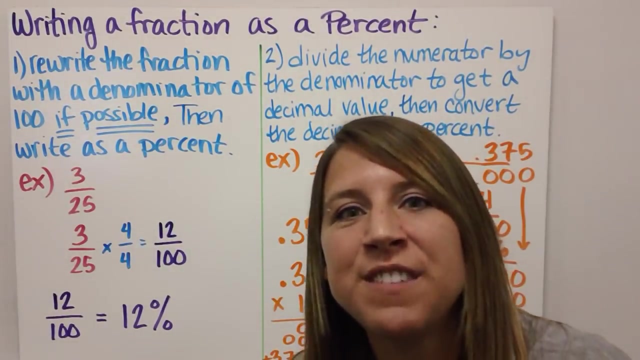 to 12 percent. Awesome, Love that method. But sometimes you may have a fraction that doesn't have a denominator that evenly goes into 100 to represent our percent that way. So you have to look at this fraction as an unsimplified division problem, which is what fractions are. 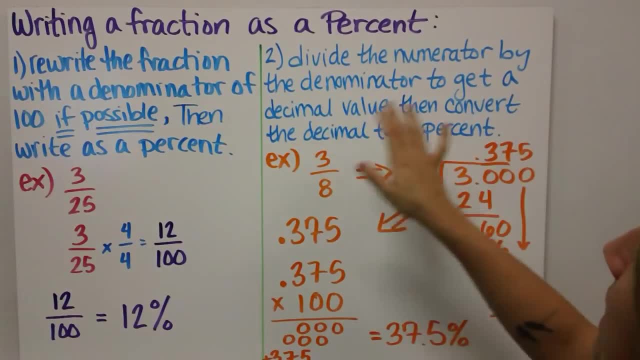 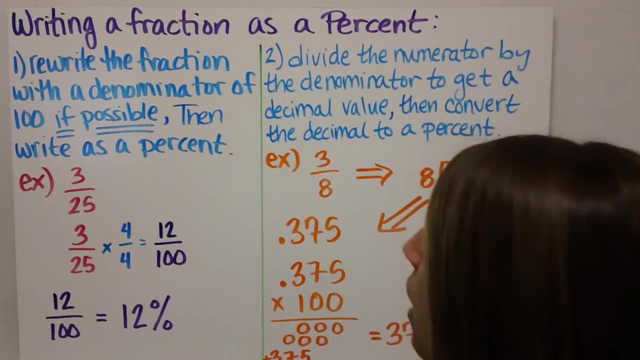 So we can divide the numerator by the denominator to get a decimal value and then convert the decimal to a percent. We should be comfortable converting decimals to percents by multiplying by 100. So if I take 3 eighths, I'm going to divide 3 by 8.. That's what it looks like over here: 3 divided by. 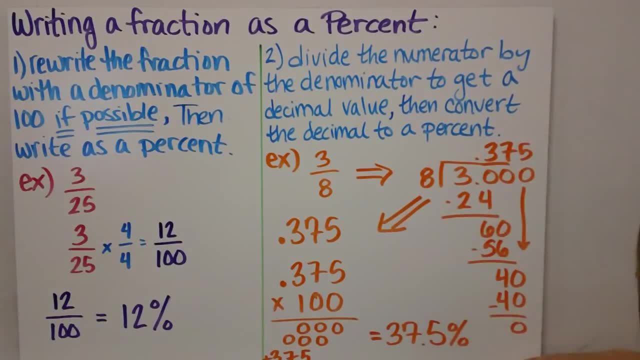 8. You know you have to add your decimal and your zeros, go through that long division. you get 375 thousandths. It's kind of wild, right, 375 thousandths. So this is my decimal value. Now I know how to turn a decimal into a percent. I multiply. 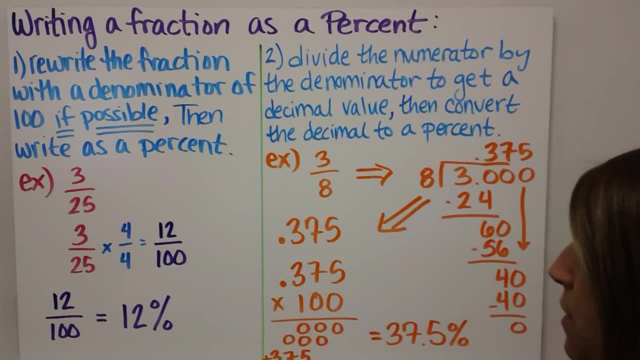 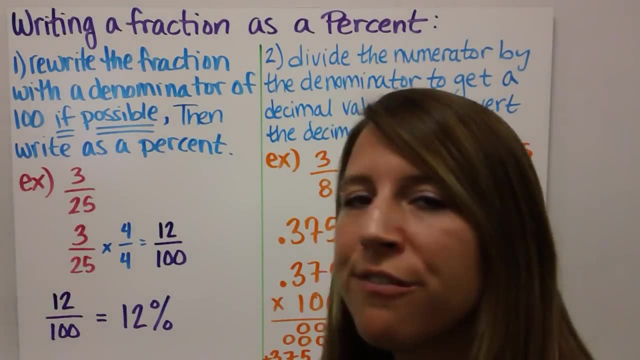 by 100, and then here I end up with 37.5.. 37 and 5 tenths percent. Okay, remember, when you multiply you don't just get 37.5.. It's representing part of a whole, so it's 37.5 percent. 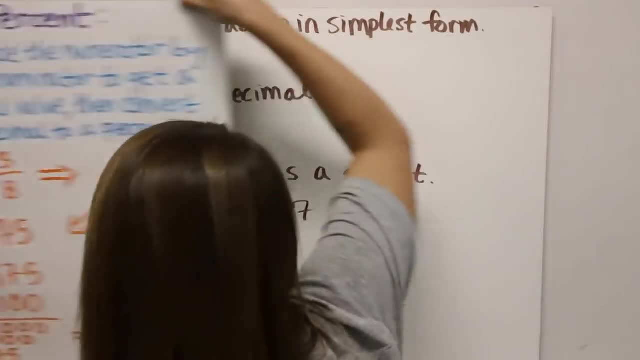 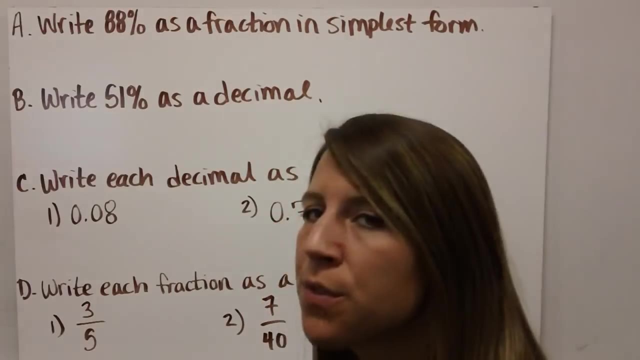 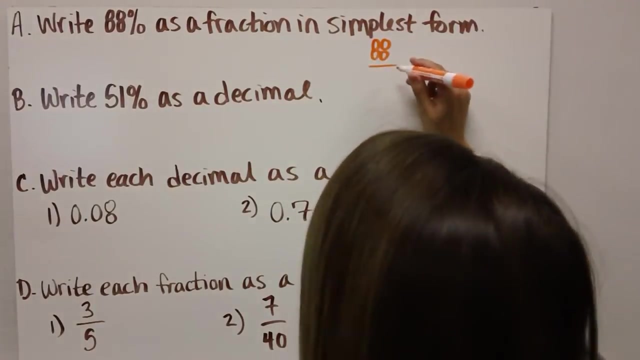 Love it. So let's work through a few of these really quickly. Write 88 percent as a fraction into the denominator. In simplest form, a percent is a comparison to 100, and so I can say: well, that's why did I do it like that: 88. 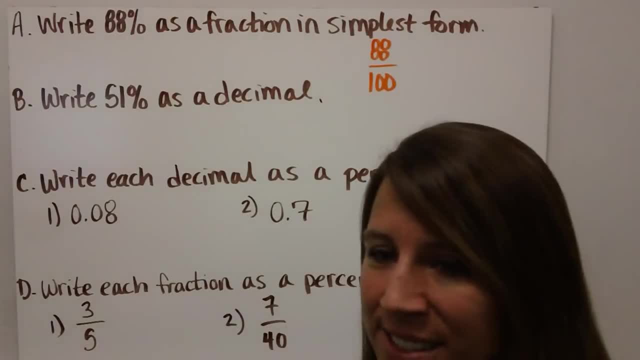 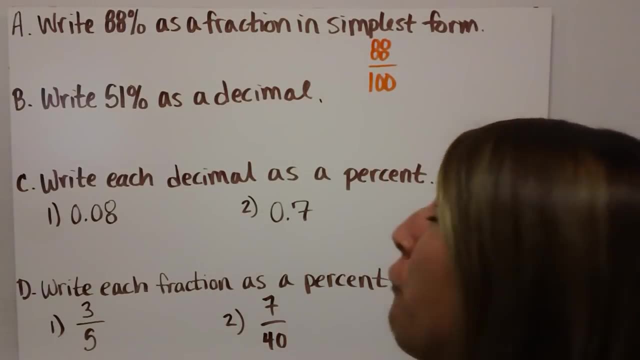 over 100, 88 hundredths right, 88 percent. But then it says in simplest form: So I can tell you that I think 4 goes evenly into both of these. So I'll just simplify by dividing by. 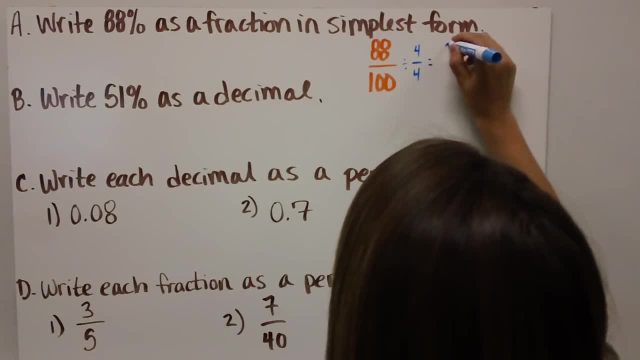 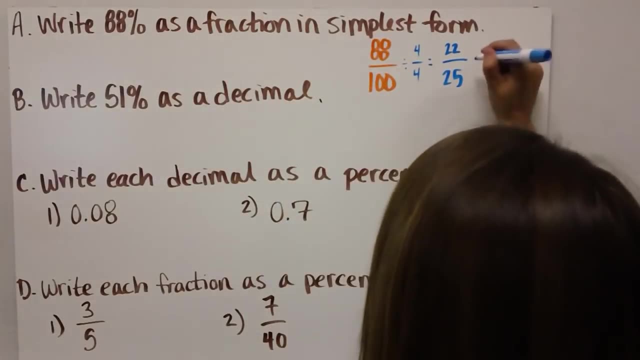 4 fourths, That's going to give me 2- twenty-fifths. Can I simplify that any further? I don't believe I can, so that would be my fraction in simplest form. How about write 51 percent as a? 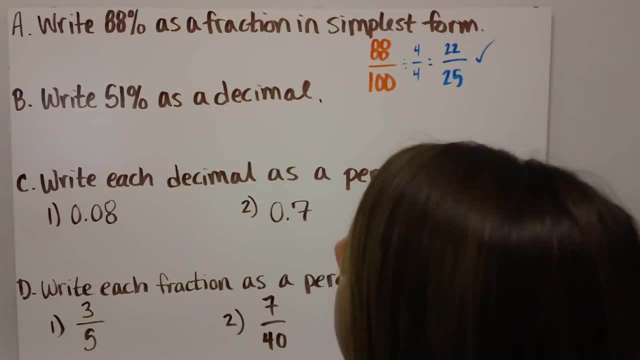 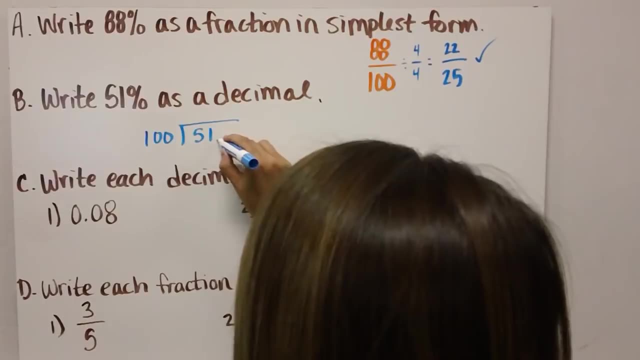 decimal. How do I turn a percent to a decimal? I divide by 100. So 51 divided by 100. I'm going to have to put my little decimals there. 100 goes into 500. five times That's 500.. 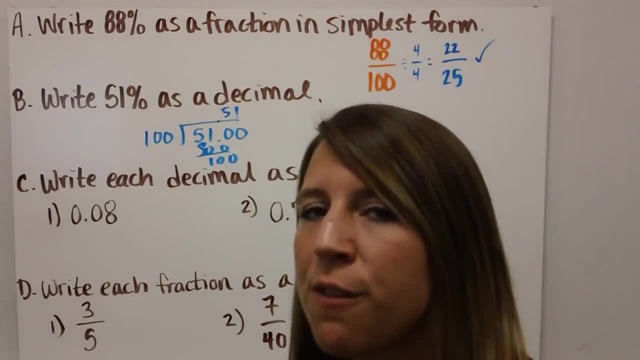 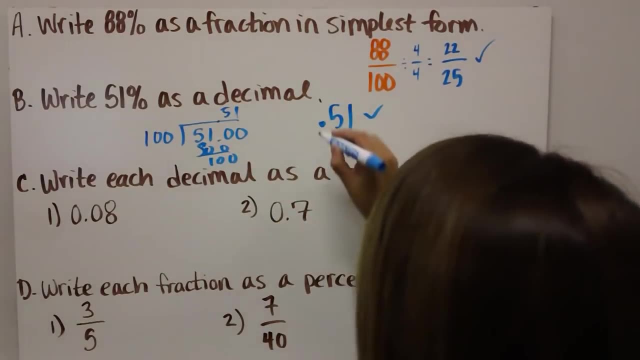 100 remains. That's going to go in once. So 50 one hundredths. You may be seeing that pattern now if you haven't seen it yet. So 50 one hundredths is my answer If you want to put that zero. 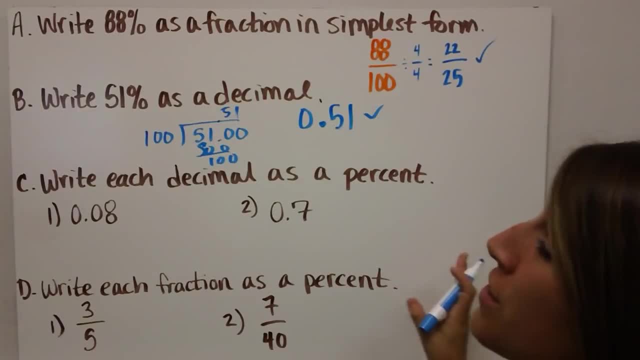 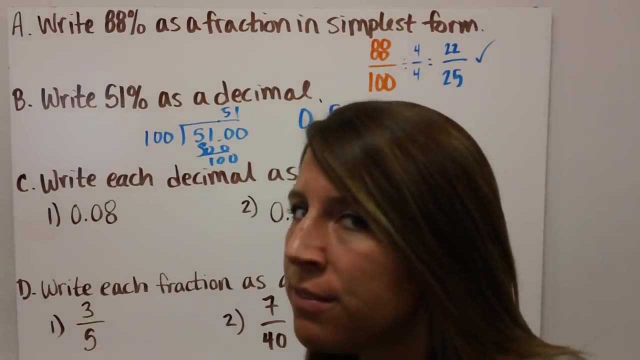 there you can Write each decimal as a percent. So to change a decimal to a percent, I multiply by 100.. I'm going to show you the pattern here in just a second, But I want to do the math first. So if I'm multiplying by 100, I'm going to 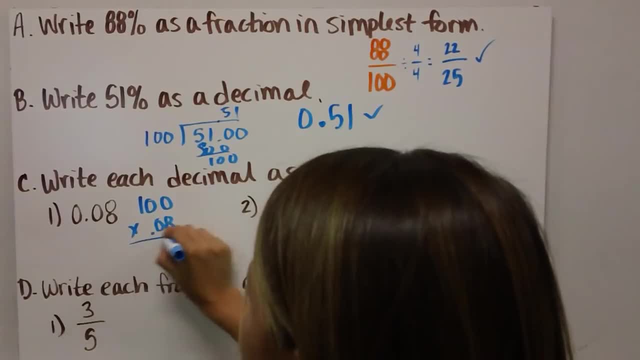 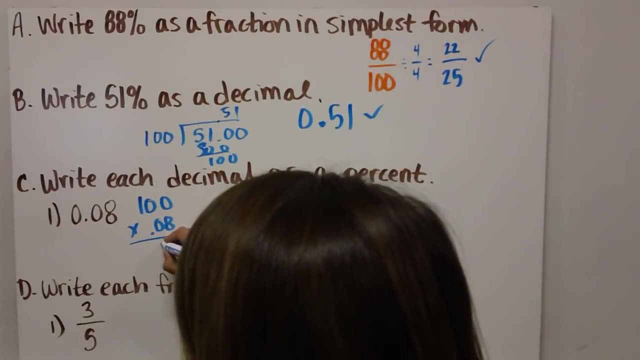 say: well, 100 times .08.. Remember, it doesn't matter which one goes on top and which one goes on the bottom, because of the commutative property of multiplication. So that's going to be 008, and then zeros across the bottom. 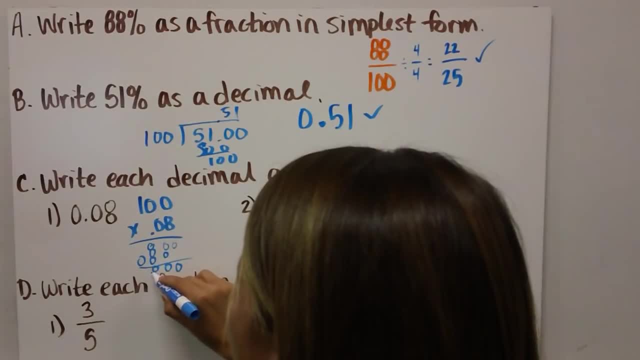 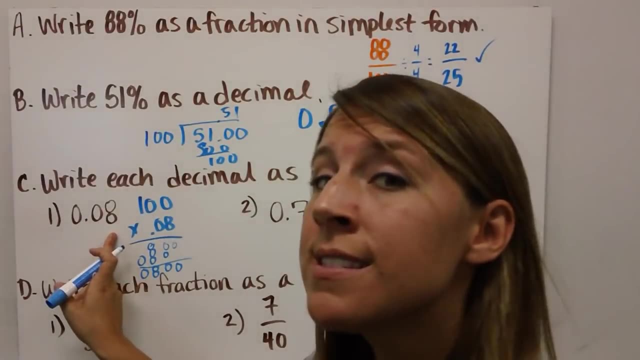 That's a zero. If I add it, it's 0080 in two decimal places. That gives me 8.. So to get from eight hundredths as a percent, that's 8%. Think about that. Eight hundredths. Well, yeah, of course. 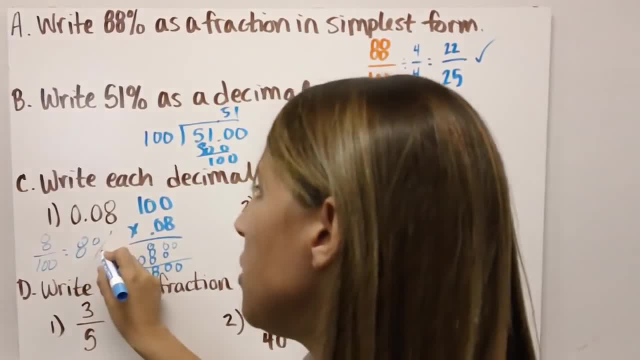 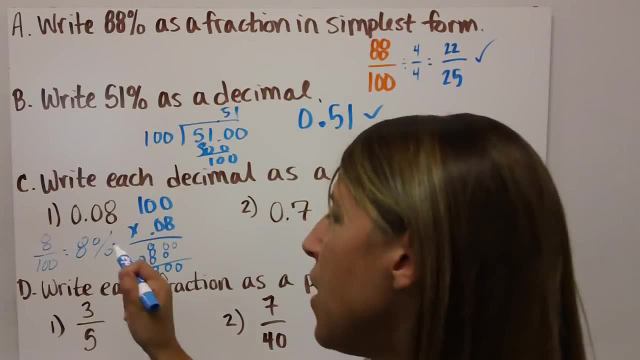 That's eight hundredths, which I know is 8%. I probably should have just done it that way in the first place, but I can also multiply by 100, which is what I did. If you have noticed- maybe, maybe not- there is a decimal. 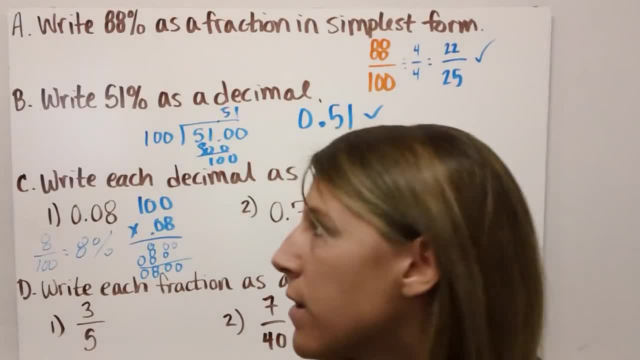 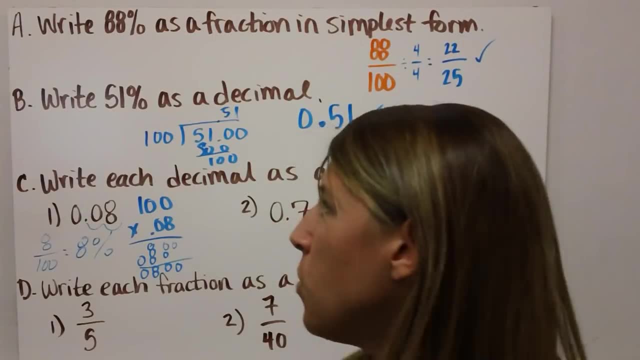 movement pattern. but I want you to understand why the decimal movement works the way it does. So to change a decimal to a percent, you can just move that decimal two times to the right and you will get the correct percent. So like here: 7 tenths as a percent You do have. 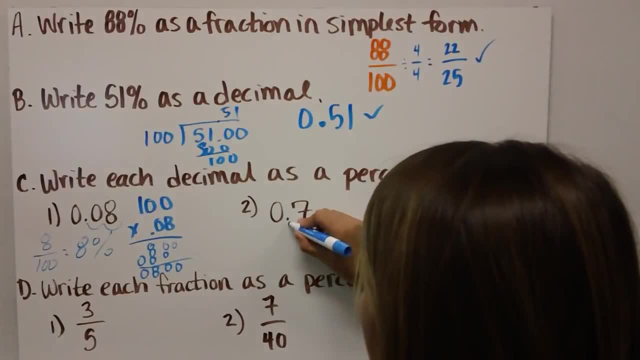 to move it twice, because it is a multiplication by 100.. If I move it twice, though, you're going to run into some problems when you run out of digits. There's nothing here, but technically there are zeros forever Right, And it doesn't actually change the value. So this 7 tenths- 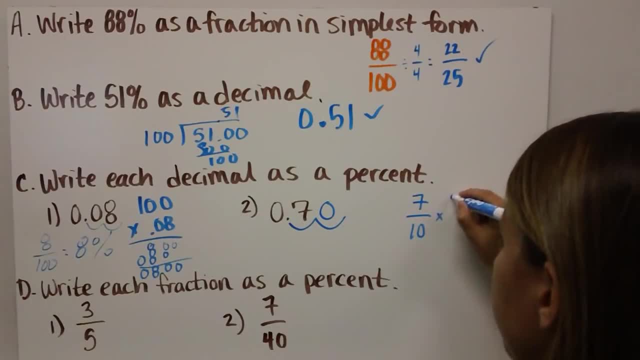 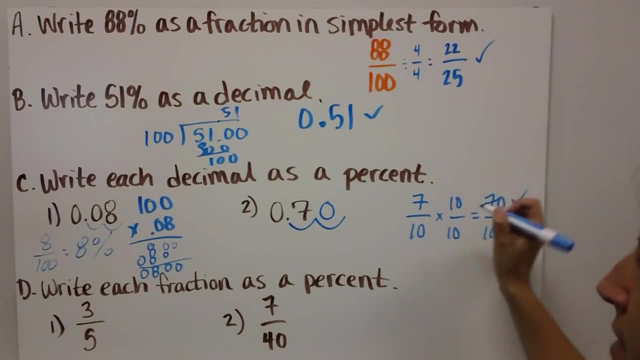 which I can say is 7 tenths. If I multiply by 10 tenths here to get that denominator, that's 70, one hundredths. This is technically 70%, right, And that's what happened when I moved that decimal twice. I multiplied by 100. 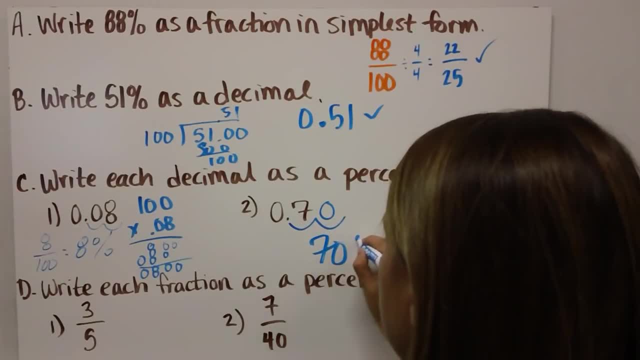 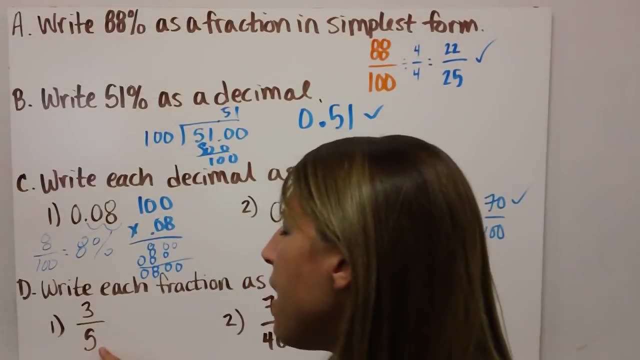 And so 7 tenths turns into 70%, which is pretty awesome. I can dig it. How about write each fraction as a percent? 3 fifths 5 goes evenly into 100, and I like that method quite a bit. So to turn 5 into: 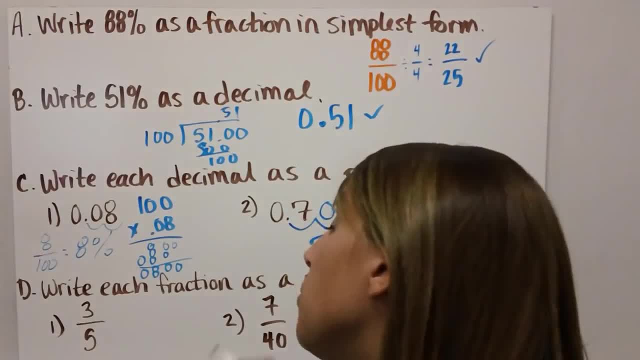 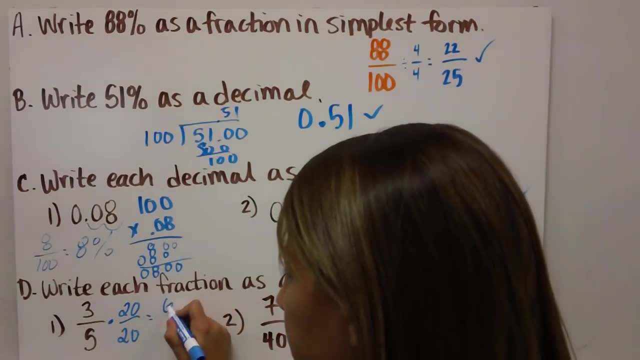 100, I know that it goes in 20 times, so I need to rewrite my fraction multiplying by 1 as 20. twentieths 3 times 20 is 60 over 100.. 60 hundredths is 60%.